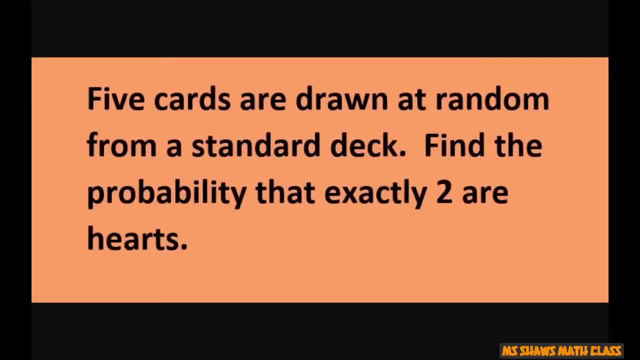 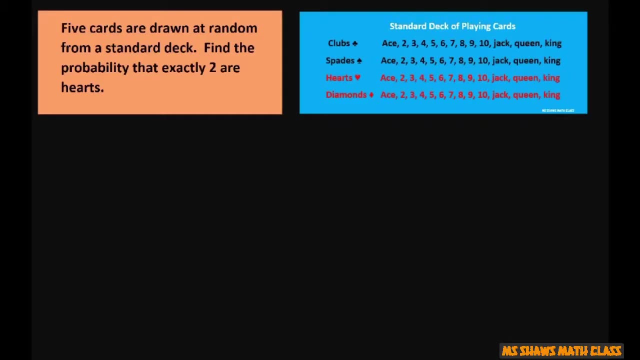 Hi everyone. Five cards are drawn at random from a standard deck. Find the probability that exactly two are hearts. So for this one it's impractical using a card-by-card approach like we did in the previous video. We don't know if the hearts are going to appear on the first or second cards. 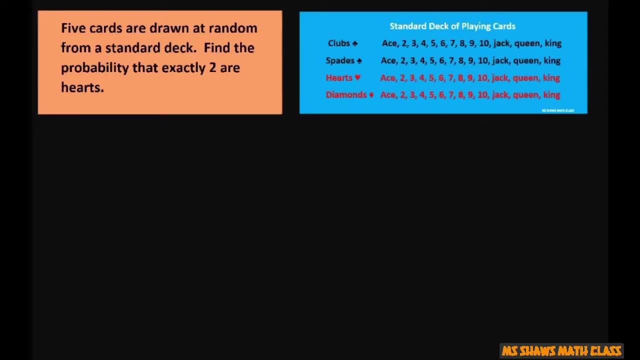 So the best way to do it is to do the second method that we used. So, for example, we're choosing two are hearts, So there's 13, choosing two for the two hearts. But again we're choosing five cards, So there's 39.. 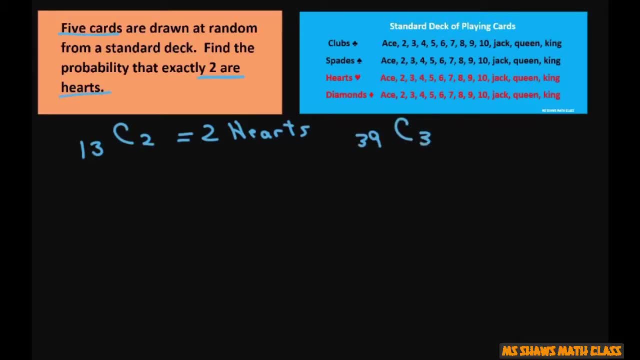 And we're choosing three for the other three cards. So by the multiplication principle that we used earlier, we're going to do the probability of two hearts and three non-hearts. So this is going to equal 13. choose two times and we have to do our. these are non-hearts, our non-hearts. 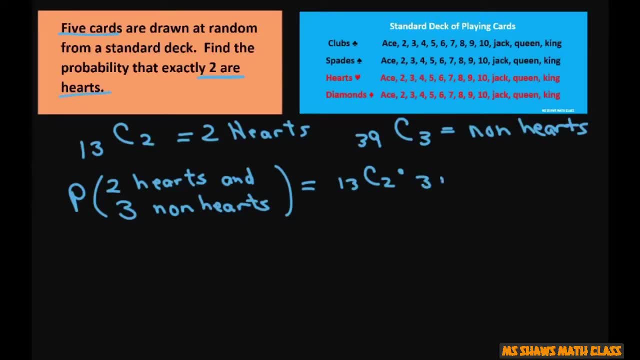 Our three non-hearts are going to be 39. choose three. Now that's going to give us our total is: we're choosing five out of the 52 total, So your total line always goes there. Now, simplifying this, we get 79 or 78 times 9,139 divided by 2,598,960,. 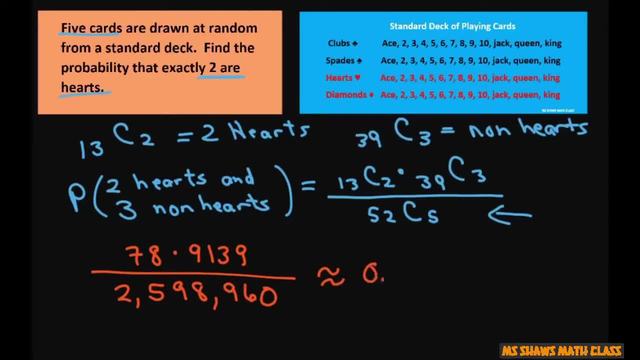 which is approximately 0.2.. 2,7,4.. And, and remember, what we have here is this: 13 plus 39 equals the 52. So we're choosing two out of the hearts and three out of the remaining 39..